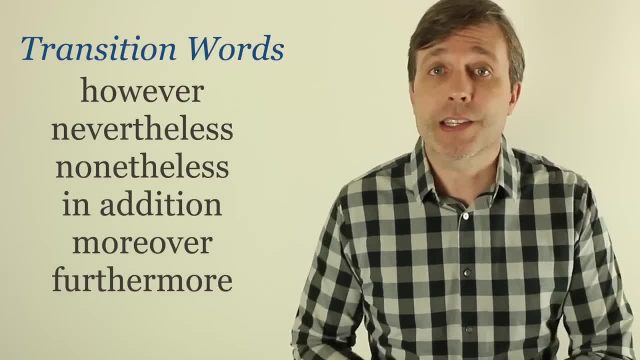 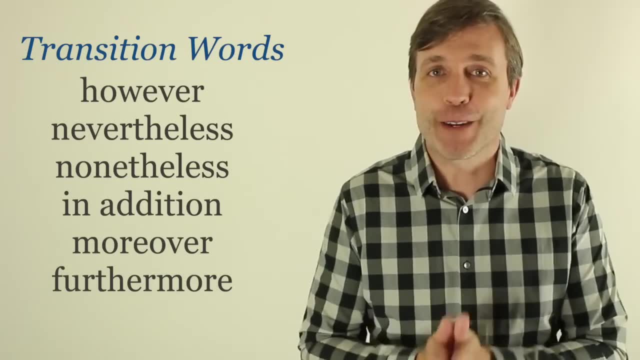 words. They are all adverbs and we use them quite often because they make our speech and our writing much easier to understand. So let's- well, let's- make it easier for you, because right now I want to put them in groups. So we have two groups and that first group. 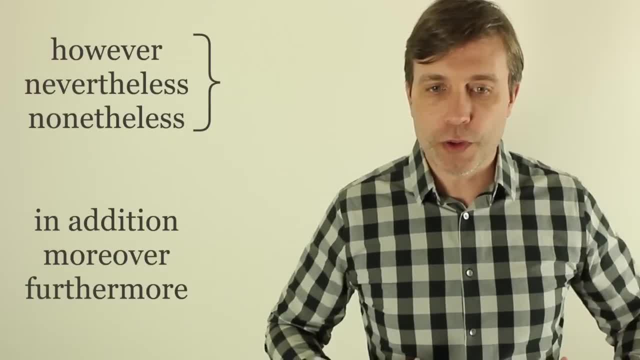 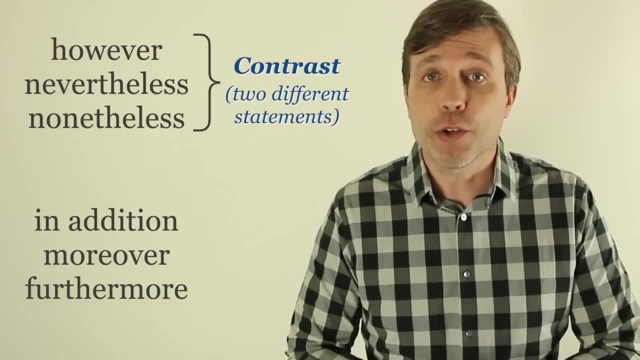 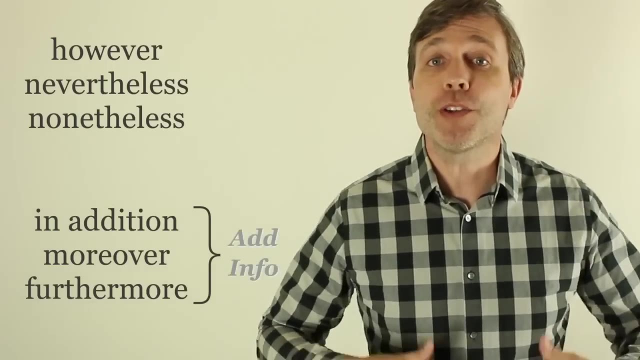 however, nevertheless and nonetheless, those adverbs are used to contrast two sentences, and you're basically emphasizing how two statements are different. The next set, which is in addition, moreover, and furthermore, are used to add information. You're adding information to something that was previously said. Now, often these words, 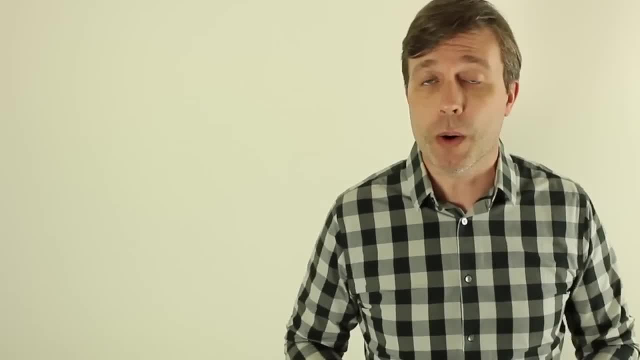 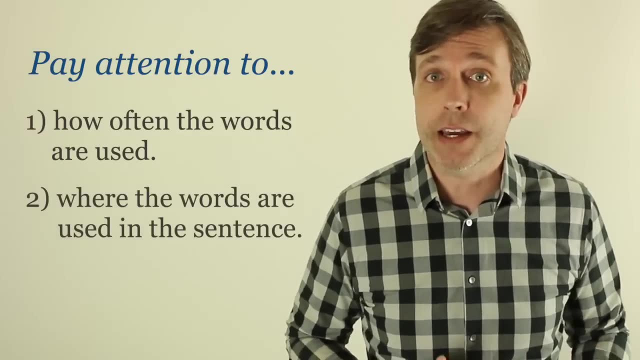 are interchangeable, but it's very important to know well how often we use these different words, where in the sentence you can use them and if that changes the meaning at all, as well as any of the slight differences between these words, which there are some, and I will. 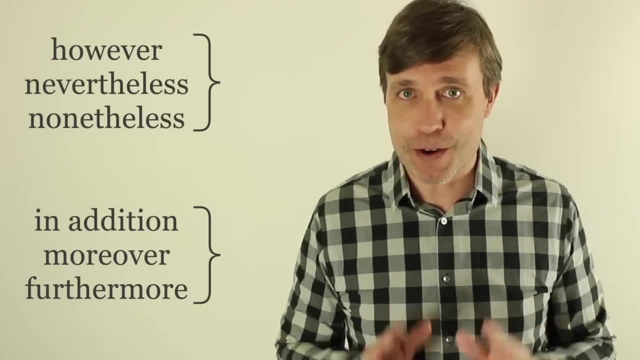 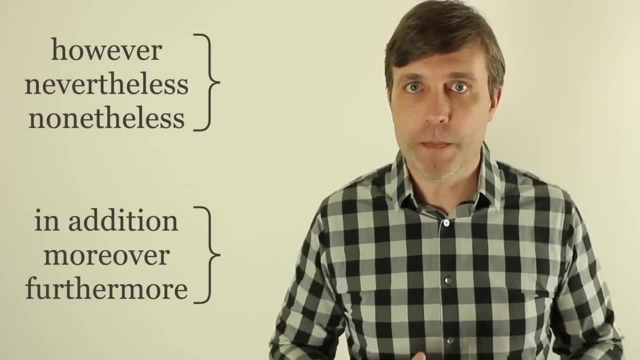 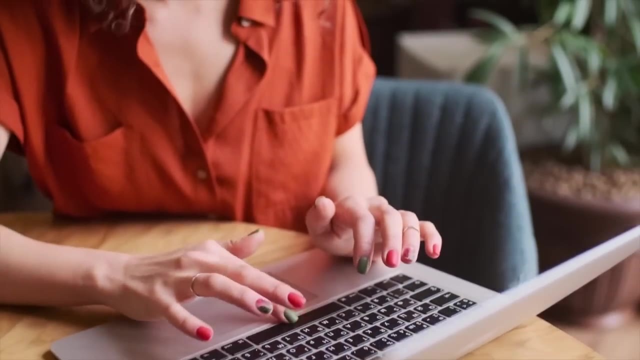 get into that a little bit later. The one thing I hope that you notice, even though these words may be interchangeable- is that I continue. I continue to use different ones, and that's really important, because when you are you're speaking and giving a presentation, or if you're writing an essay, it's likely that you will. 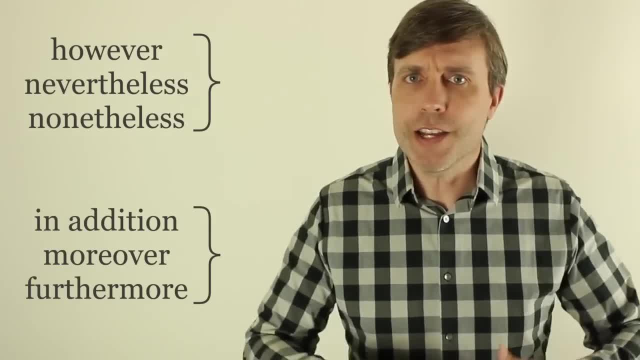 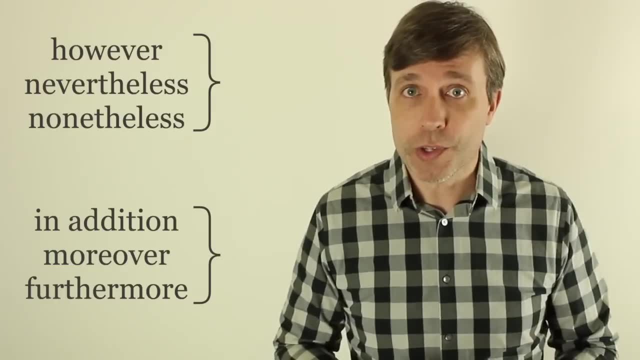 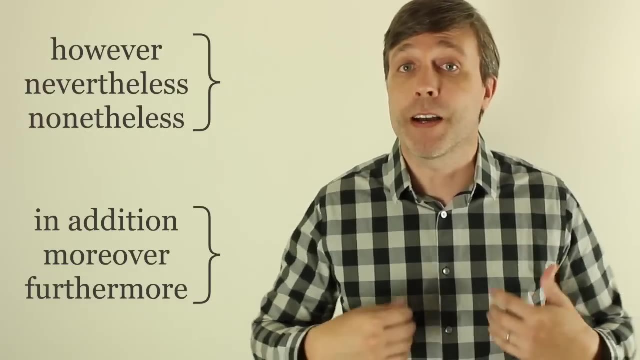 need to use transition words multiple times and you don't want to just use the same word over and over again. It's also important to know which one to use and which one is more effective, because there are some slight differences, and that's going to help you become a more effective speaker. 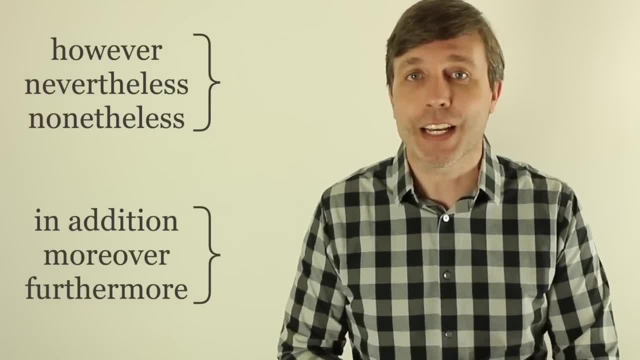 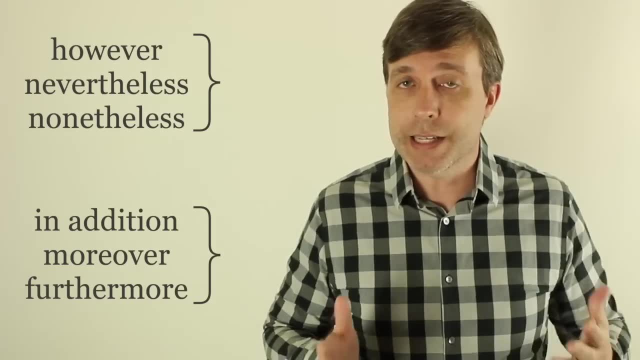 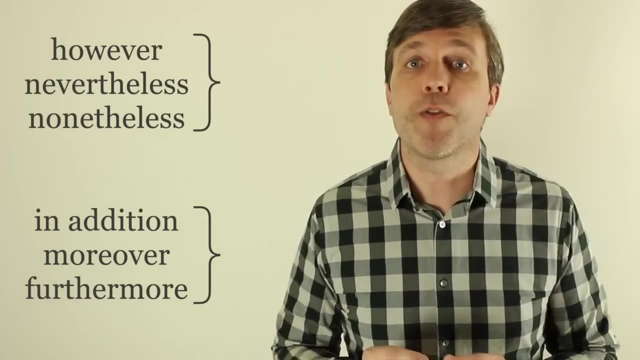 and a more effective writer, Which is how it all ties into English fluency. but one thing I want to point out is that all of these words are they are a bit more formal because, as I said, you might use them if you're giving a presentation or you're writing an essay. however, some are more formal. 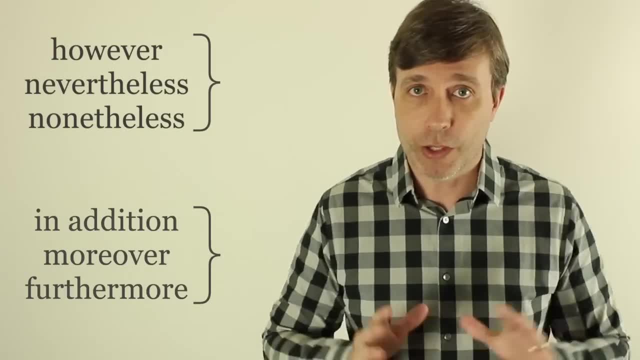 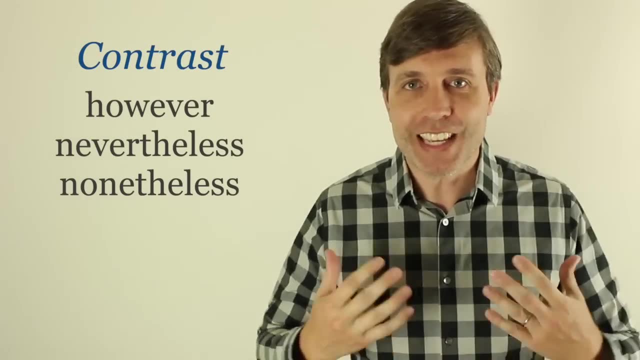 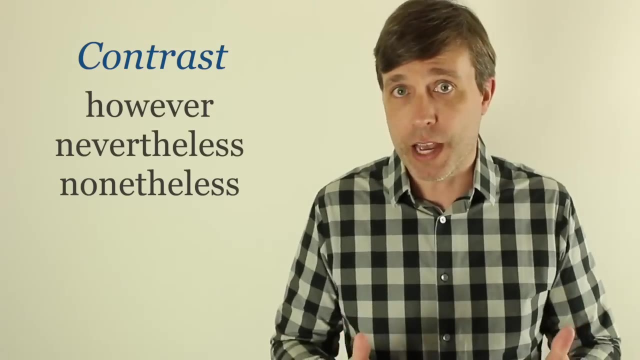 than others, and that's what I want to talk to you about right now. so let's begin with these words right here. however, nevertheless and nonetheless, these words, these adverbs that we use to contrast Two statements and say how things are different. so let me give you an example. 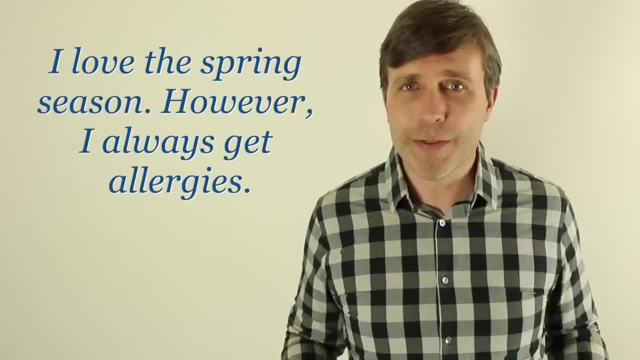 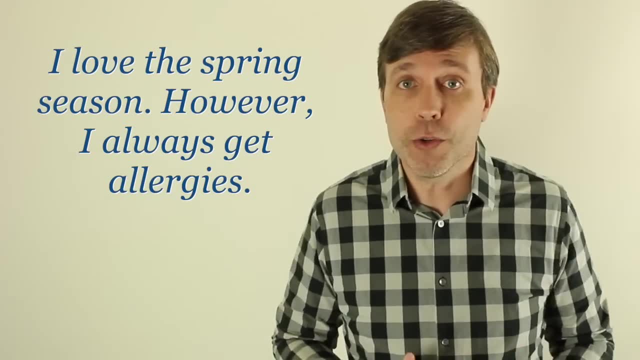 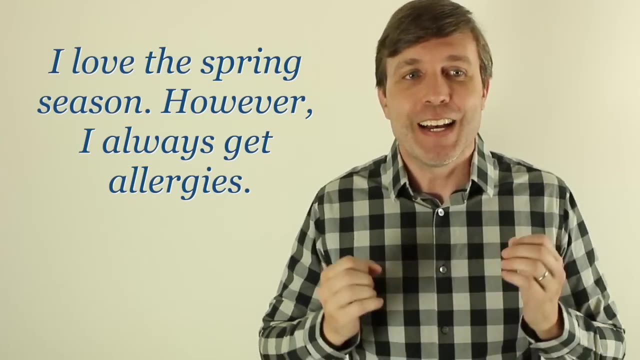 I could say I love the spring season. however, I always get allergies. alright, so I'm using, however, to contrast these two, these two different ideas, because I do, I really I love spring time. It's wonderful, It's great. 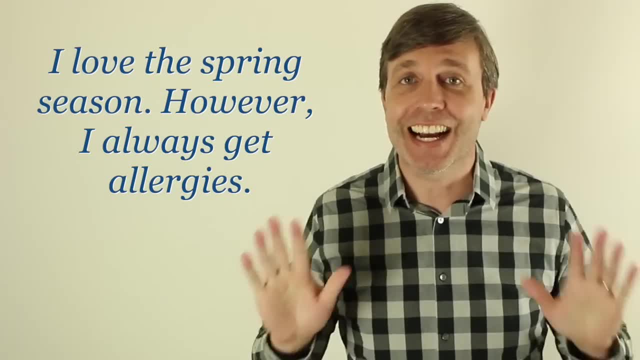 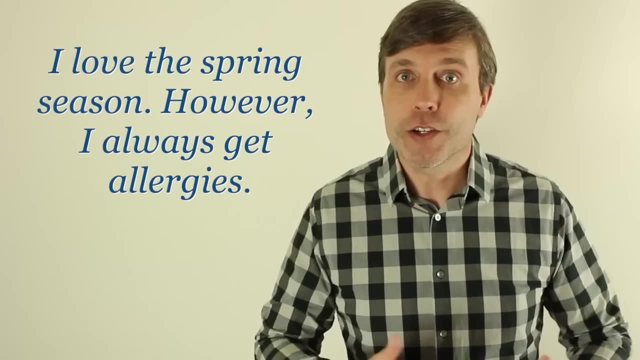 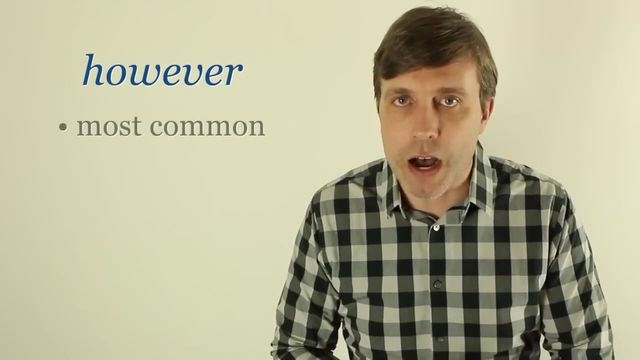 However, I get allergies. It's something that I hate. I don't like just when I'm coughing and sneezing all the time, So this is a very useful adverb that I can use to contrast these two statements. Now, I used, however, because this is- this is definitely the most common adverb that 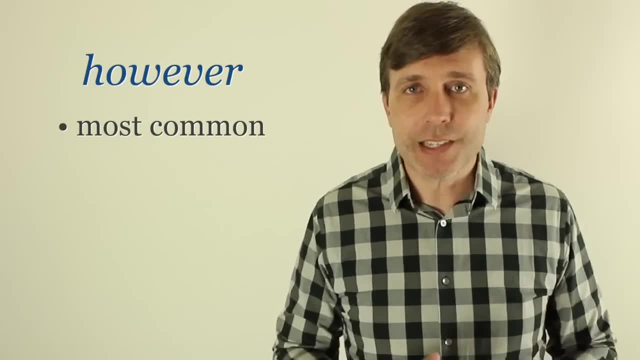 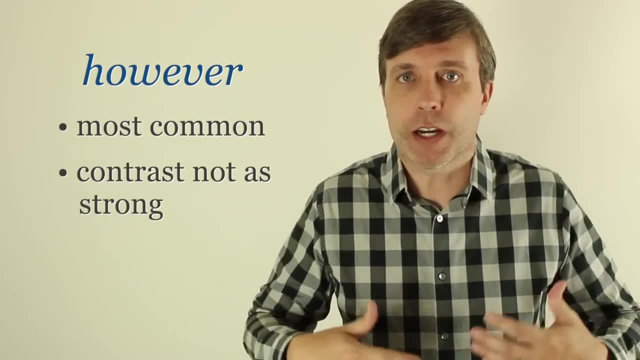 you can use if you want to contrast and because of that it's probably not the strongest as well. So in the case of we're talking about spring and allergies, it's more conversational English Now I could use. nevertheless. 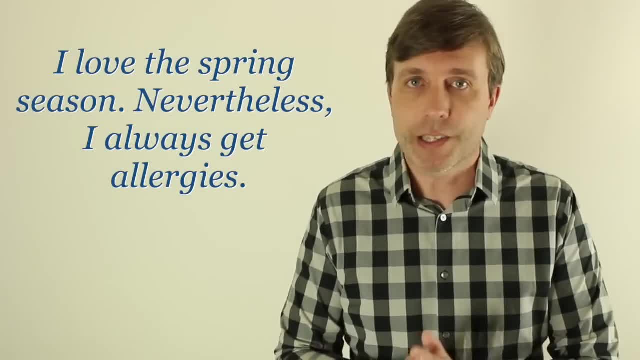 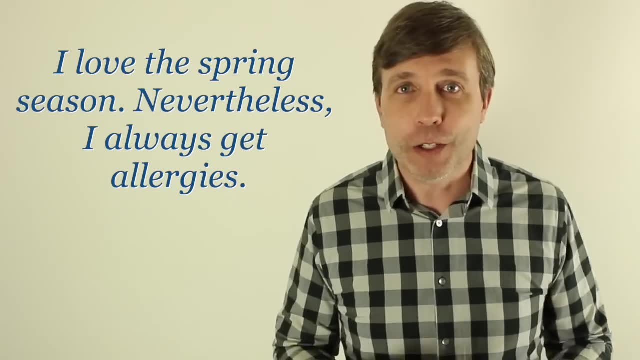 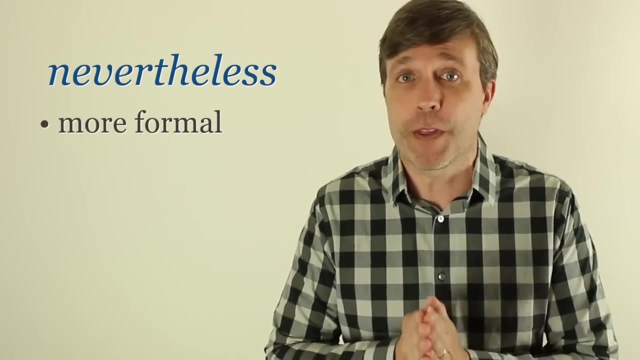 It's interchangeable. I could say I love the spring season. nevertheless, I always get allergies. Some people might think it could sound a little awkward, and the reason for that is because, nevertheless, it's more formal. It's more formal than, however, which means that it's not as common. 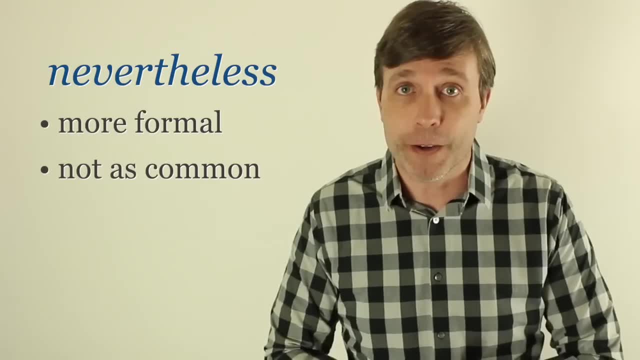 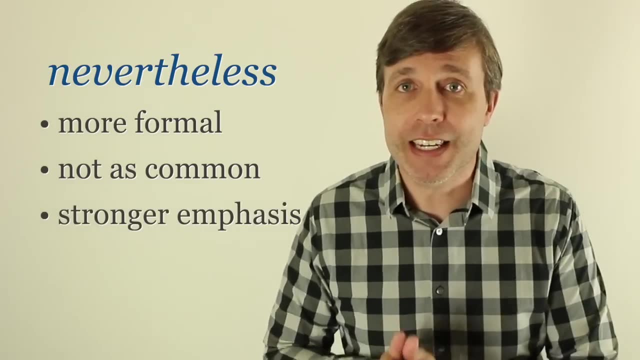 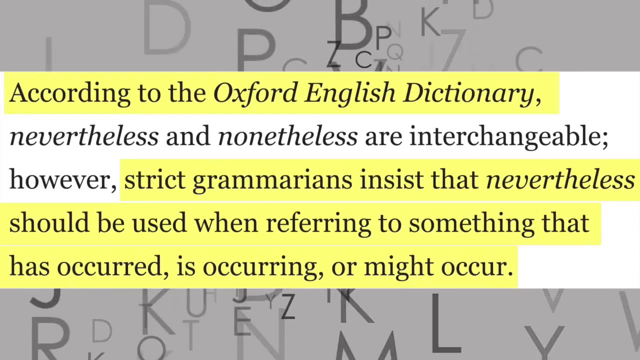 You are not going to use or hear this word as often as you would hear or use the word. however, Nevertheless, It also really emphasizes the difference, so it provides a bit more emphasis than. however, According to the Oxford English Dictionary, strict grammarians insist that. nevertheless, 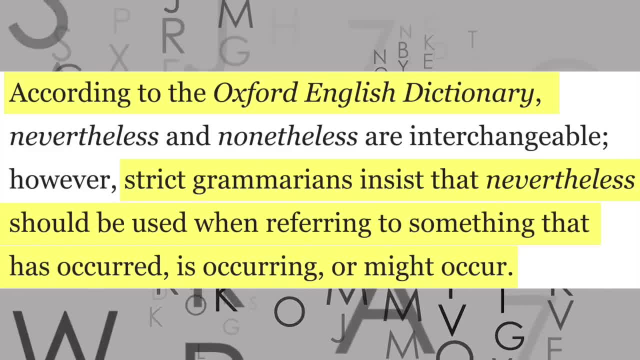 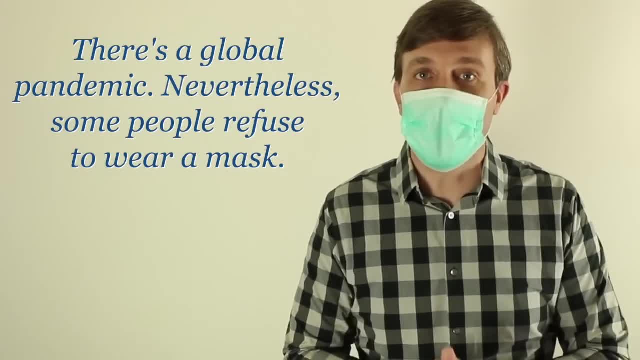 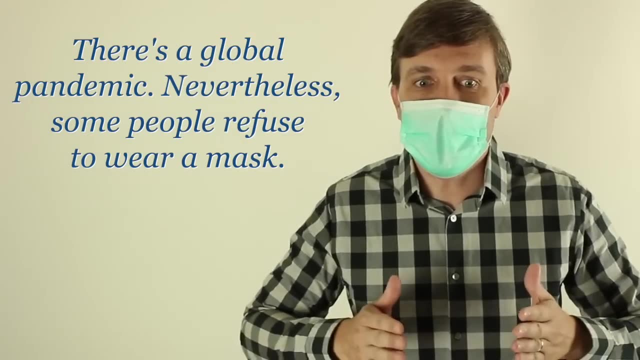 should be used when referring to something that has occurred, is occurring or might occur. Let me give you an example. There's a global pandemic. Nevertheless, some people refuse to wear a mask. So in this example we are. we're talking about something that is occurring right now. 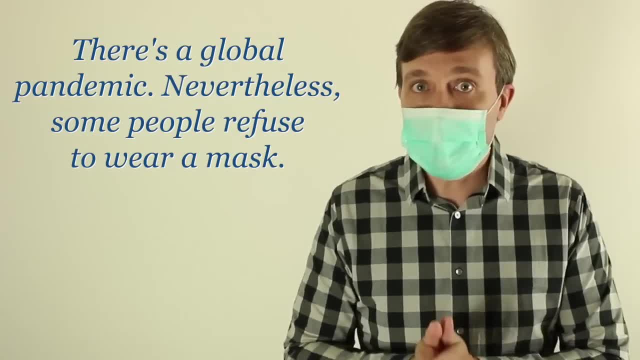 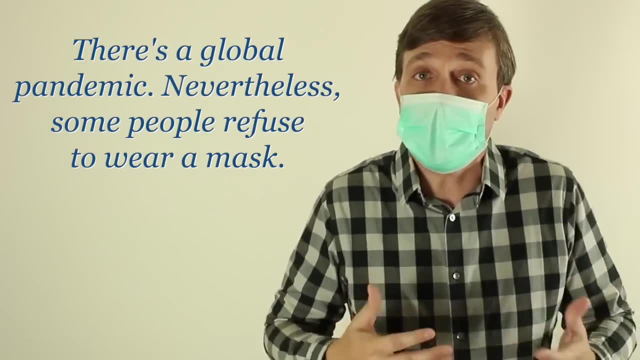 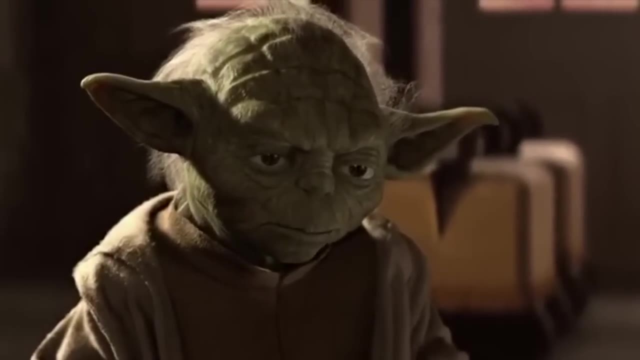 and I think it is definitely appropriate to use. nevertheless, because we're talking about something that is more formal, It's more important- and you really want to emphasize that because, yes, it's very important- that we wear a mask, The chosen one. the boy may be, nevertheless brave- danger, I fear, in his training. 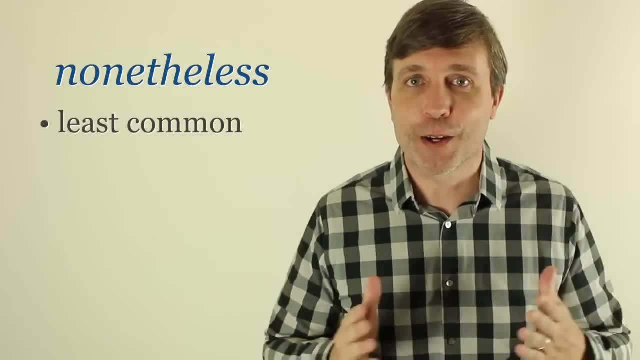 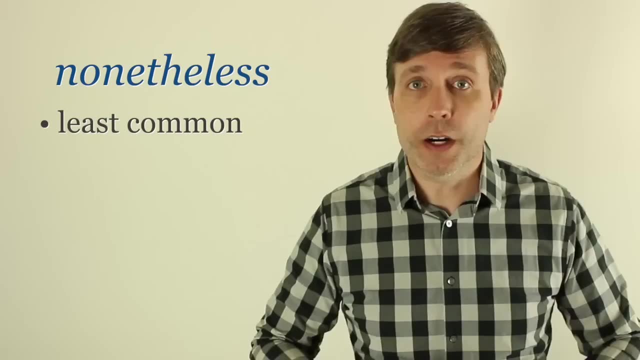 Now, nonetheless, is the least common adverb among the group and its usage has really become a little more popular In the last hundred years. So this word- nonetheless it's also more formal and you again, you use it if you. 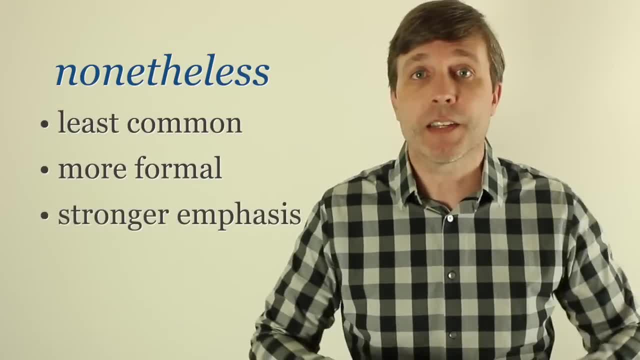 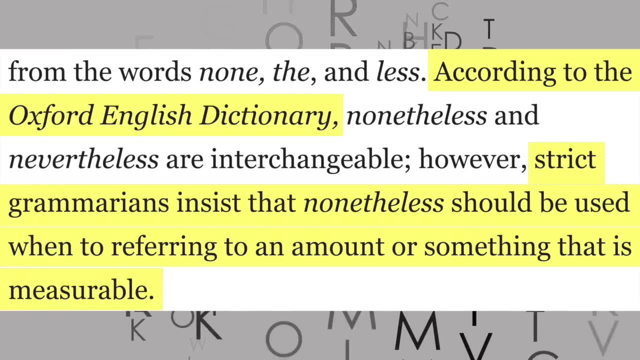 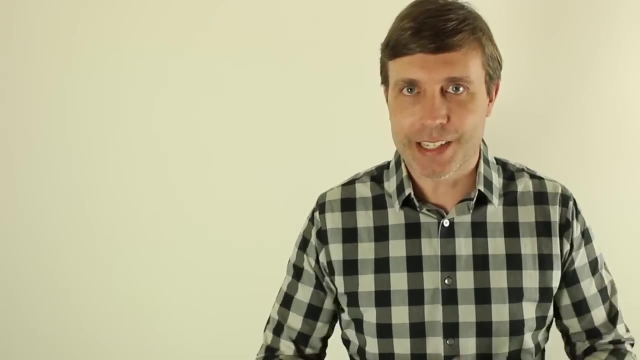 really want to emphasize the difference between two statements, But there is one slight difference. According to the Oxford English Dictionary, strict grammarians insist that nonetheless should be used when referring to an amount or something that is measurable. So I can give you an example sentence and say the business proposal seemed risky nonetheless. 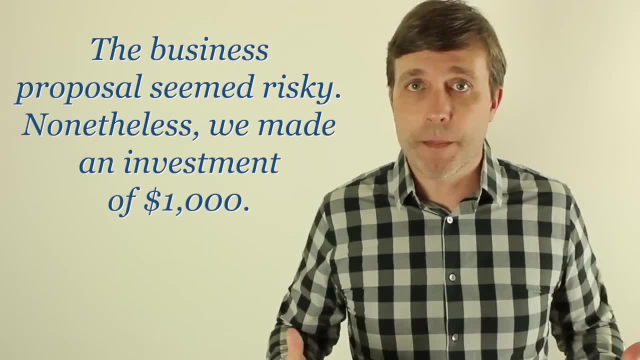 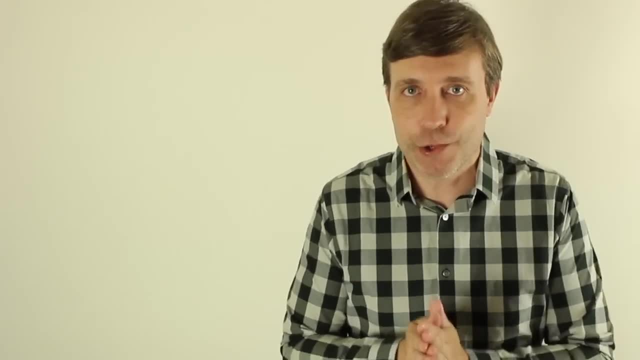 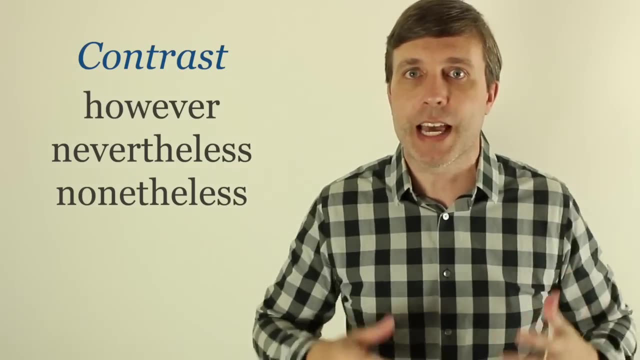 we made an investment of $1,000.. So we're talking about money and amount, and I use nonetheless Now this: this is not an established rule. Again, these words are interchangeable. The main thing that I want you to take away from all of this is that, however, is the most. 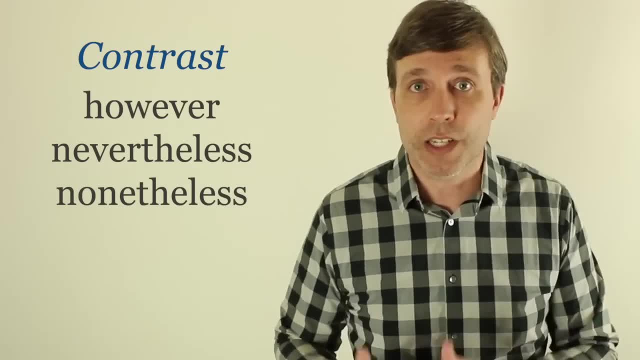 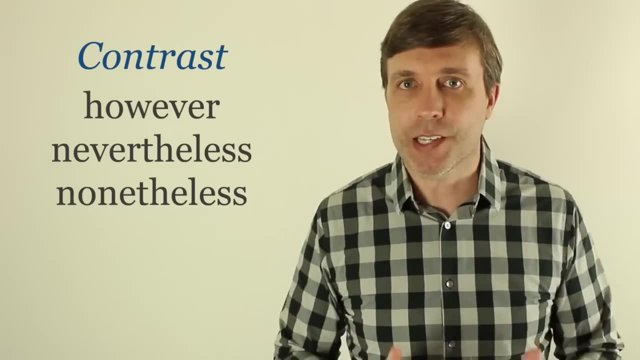 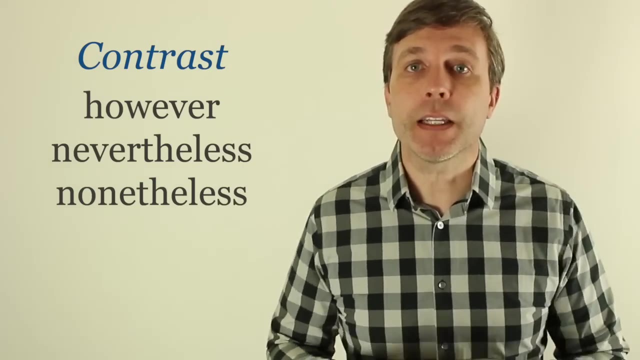 common transition word if you want to contrast two statements- And nevertheless and nonetheless, they are more formal and they are going to give a little bit more emphasis when you want to say that two statements are different. Another thing to keep in mind is that these words typically come at the beginning of a 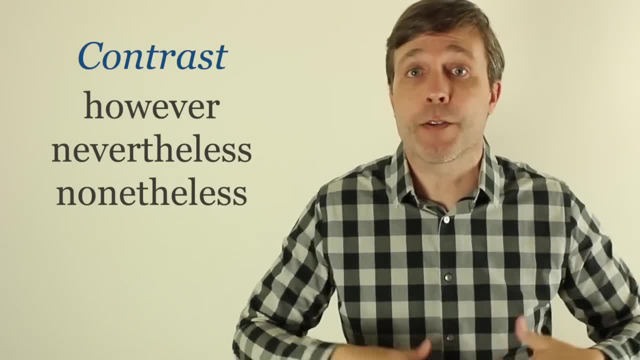 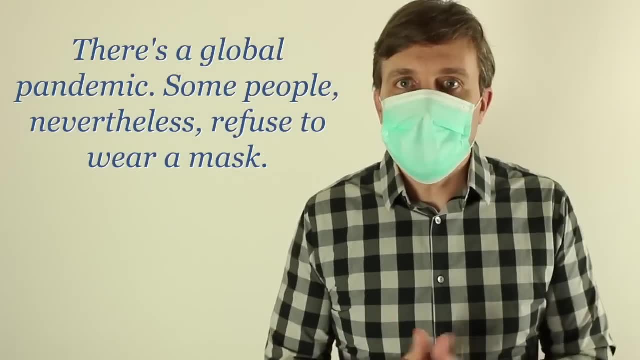 sentence, but they don't always have to. They can come in either the middle or the end of a sentence. Let's go back to some of those examples that I just talked about. There's a global pandemic. Some people nevertheless refuse to wear a mask. 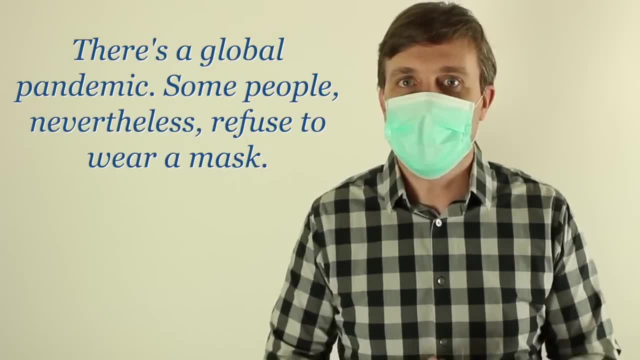 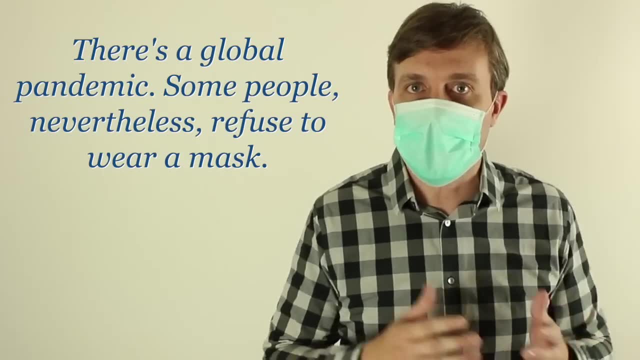 So in this case you will need two commas around the adverb so that the punctuation is correct. But if you are, if you're wondering, well, what? what's the difference between using it at the beginning or in the middle? I would say that it's not as strong that if you're. 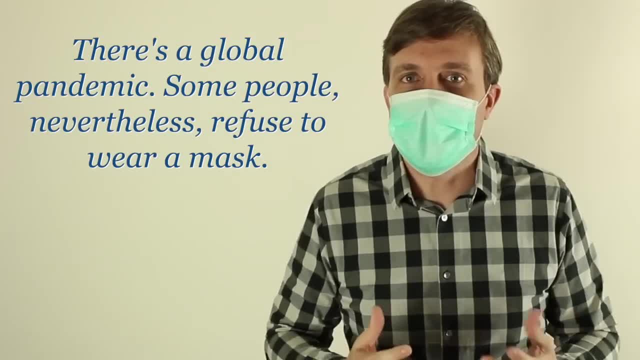 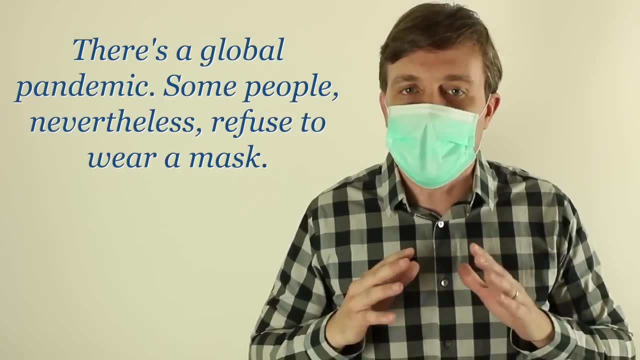 putting the adverb at the beginning, you're giving that difference a little more strength. in this case, putting it in the middle, you're you're kind of saying it as a matter of fact. you're not really trying to highlight that there is such a huge difference. 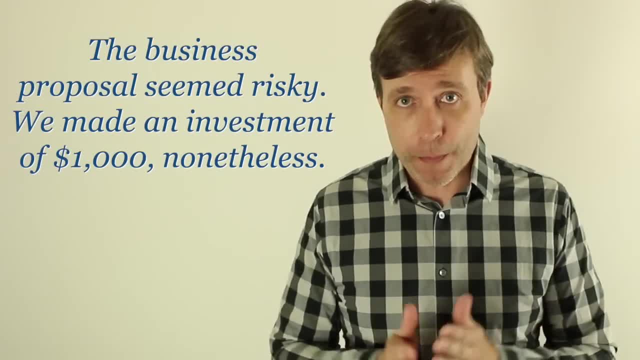 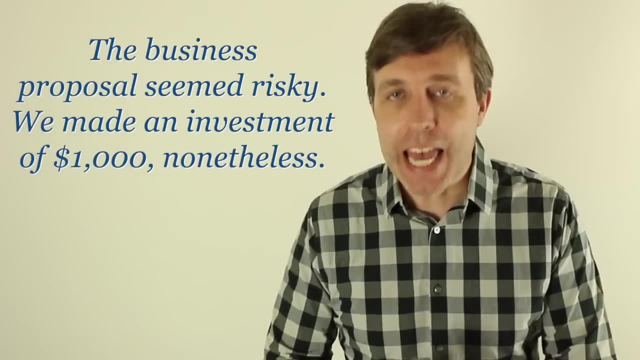 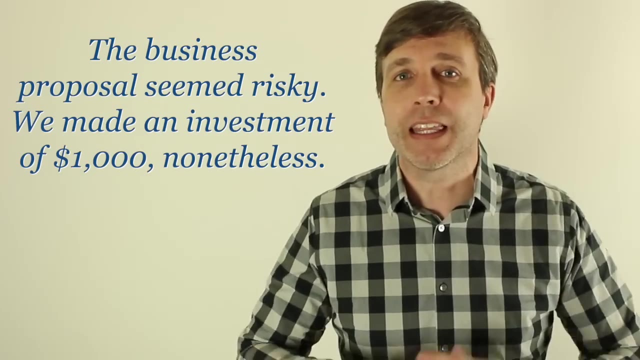 Or I could say the business proposal seem risky. We made an investment of a thousand dollars. Yeah, Nonetheless, All right. So here I put, I put the adverb at the end of the sentence And again, in this case, I think it's not as strong and this would certainly be less common. The reason why I think people will do this, especially in their writing, is more for just sentence fluency, because you want to structure your sentences in a variety of ways and you may not always want to put the adverb at the beginning. It's good to to switch things up now and then. 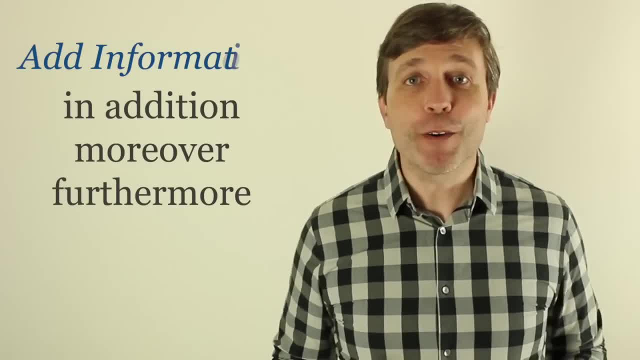 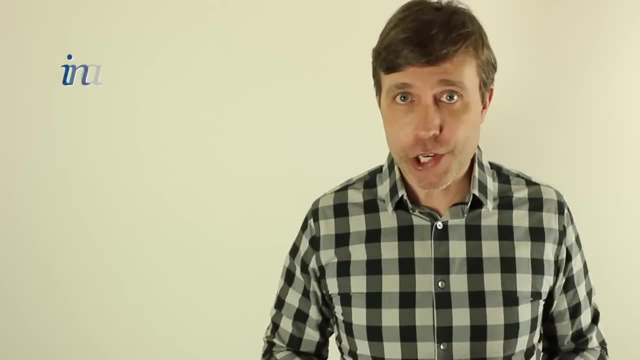 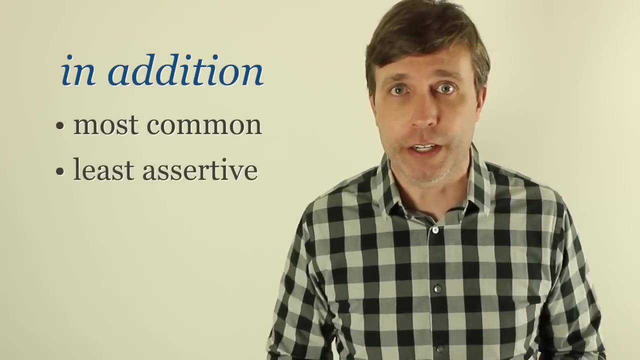 It makes reading more interesting. Now let's look at in addition, moreover, and furthermore, So these words are used when you want to add information. In addition is the most common one, And because it's the most common, I also think it's the least assertive of the three. 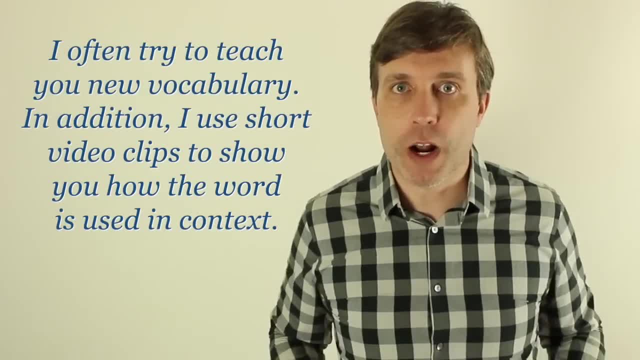 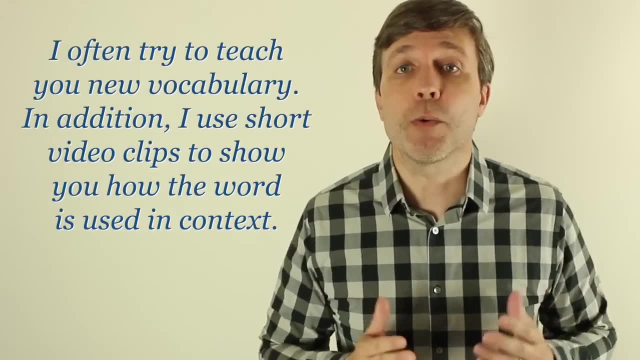 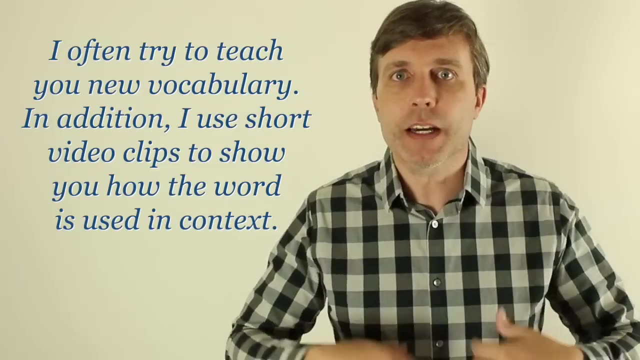 So let me give you an example. I can say: well, I I often try to teach you new vocabulary. In addition, I use short video clips to show you how the word Is used in context, So I'm adding information to what was already said. in in a way, I'm really complimenting. 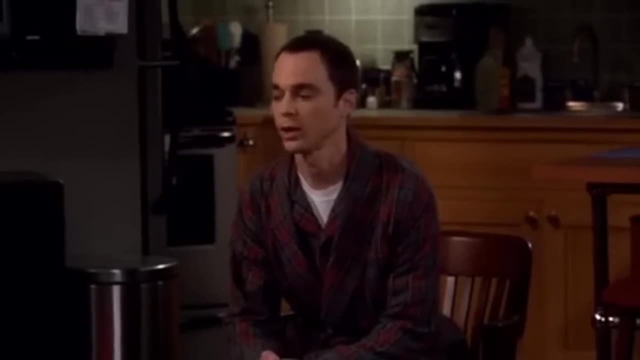 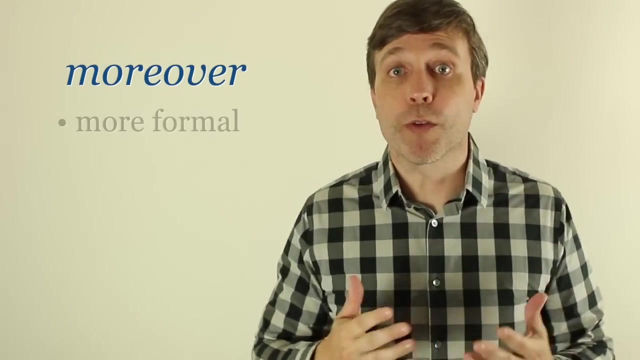 the information that I already gave you, that failure clearly stands on its own. Thanks for pointing it out. In addition, your premise is flawed. Now, moreover, is well, it's more formal, it's less common and it really adds emphasis on 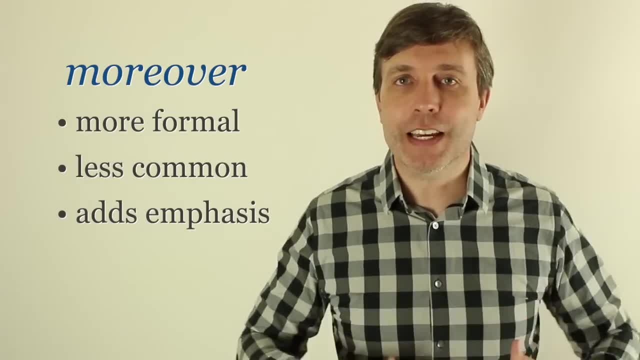 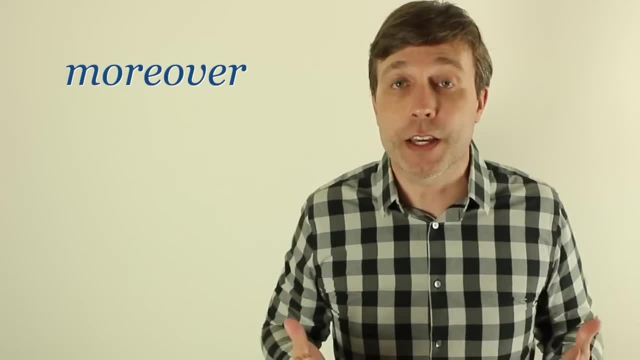 on top of what you already said. So in this case, I think it's great If you are trying to be persuasive, Yeah- And you want to build on top of something that you you said previously. let me give you an example. 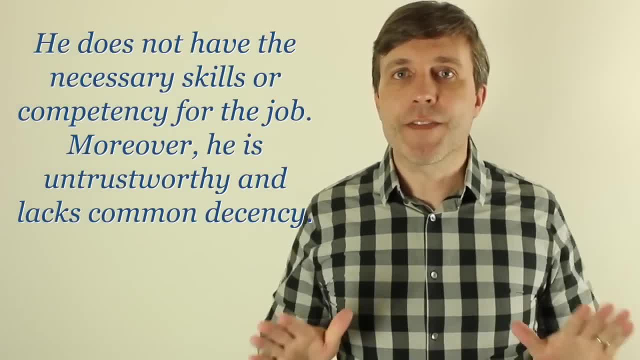 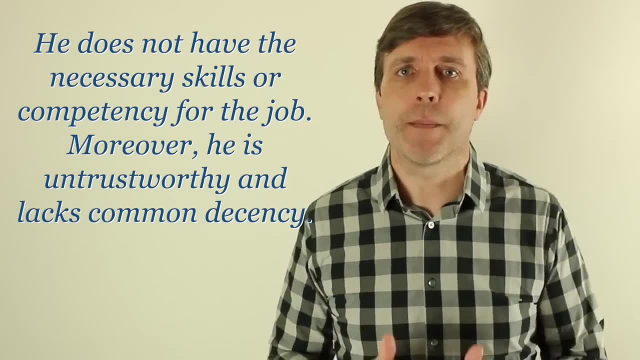 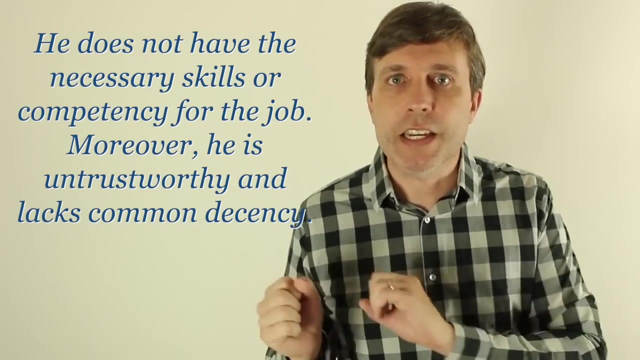 I could say that, well, he does not have the necessary skills or competency for the job. Moreover, he is untrustworthy and lacks common decency. So in this case, I'm I'm making a persuasive argument as to why, well, this person, it's. 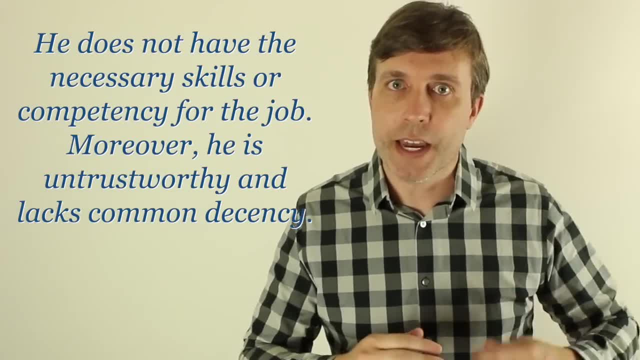 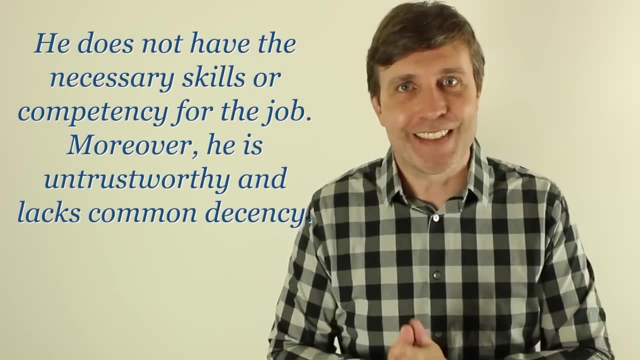 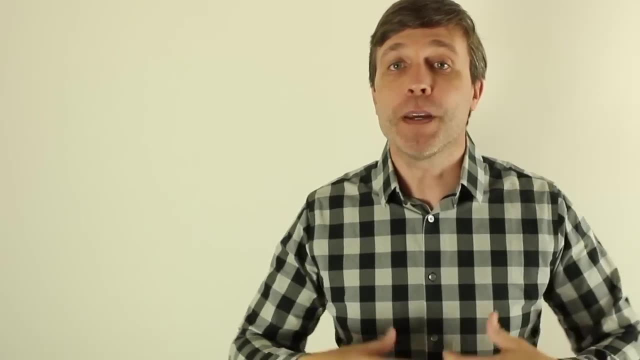 not the right person for the job, They don't have the skills. And then I build on top of that And add that emphasis and say- probably perhaps even more important- that this person is untrustworthy. They lack common decency. So in that case, if you really want to be persuasive and you're making an argument and 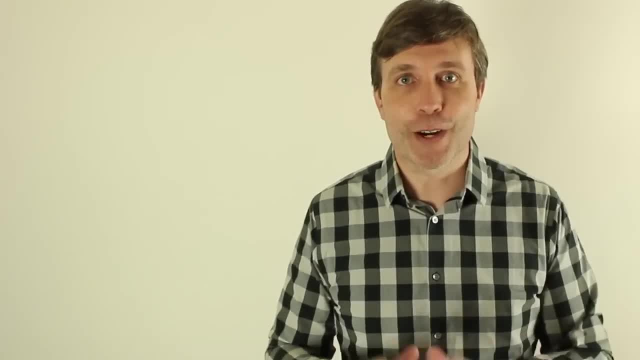 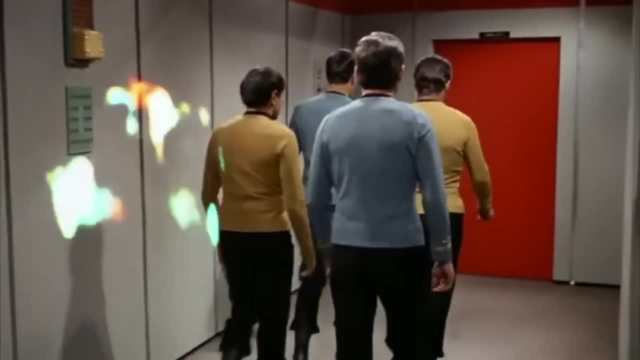 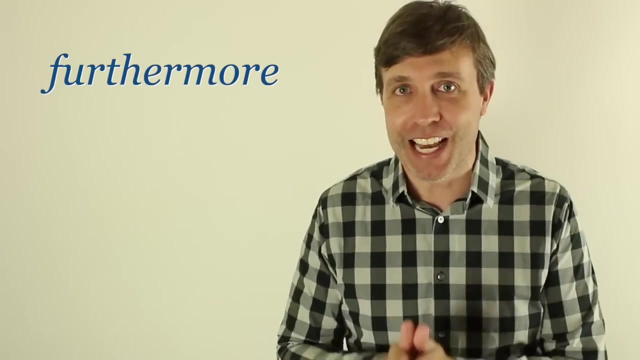 you want to build on top of it, moreover, is a great transition work. The Klingons were too far distant to have been the attackers. Moreover, they also were apparently attracted by distress call. Now, furthermore, Was a little late to the party just like. nonetheless, it's had its popularity rise. 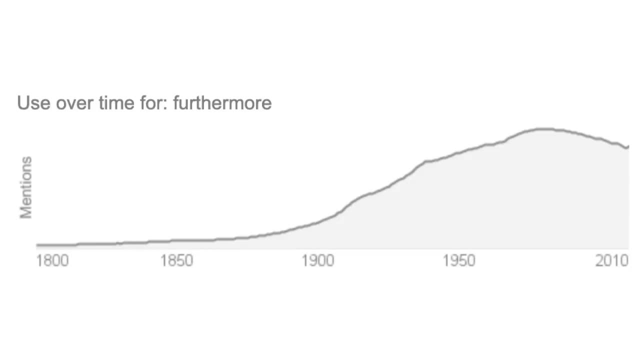 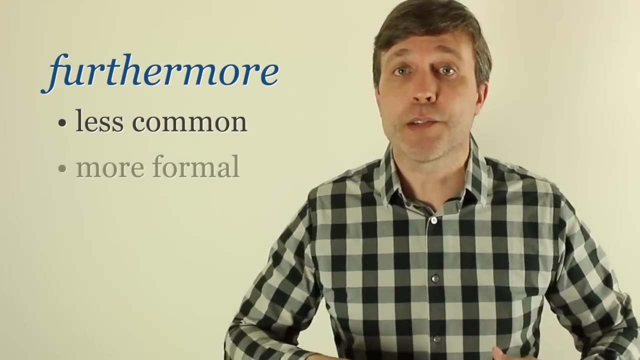 in the last hundred years, but it is. it is less common than moreover, and it is certainly less common than, in addition, but, just like moreover, it is more formal and it's going to add a bit more emphasis to the information that you're trying to add. 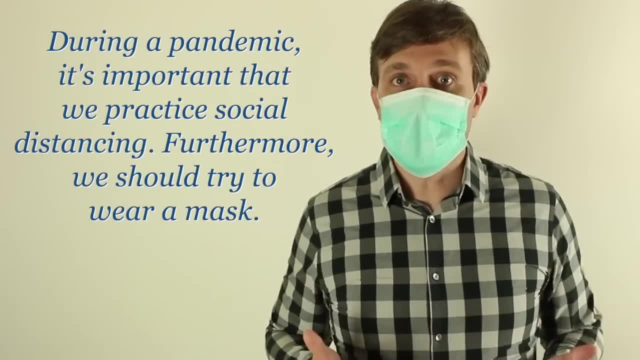 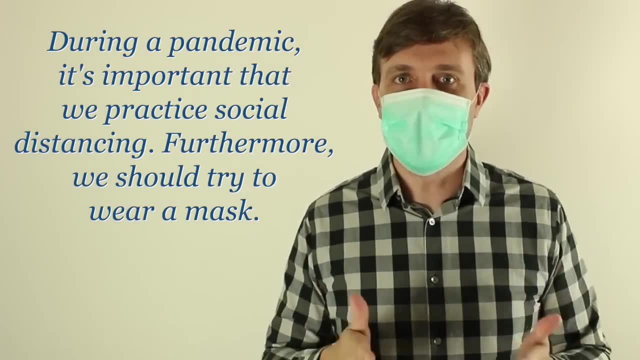 So let me give you another example. during a pandemic, it's important that we practice social distancing. Furthermore, we should try to wear a mask. right? I'm really pushing these masks on everyone, but you, you understand what I'm talking about. 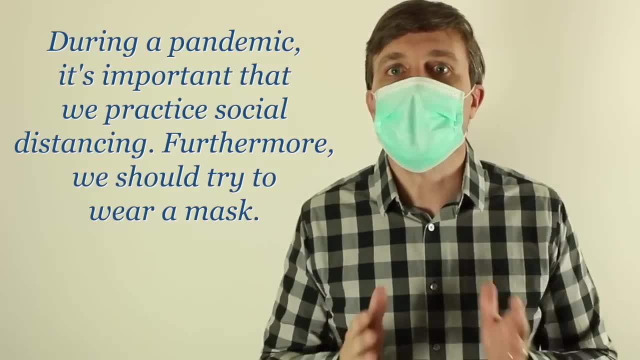 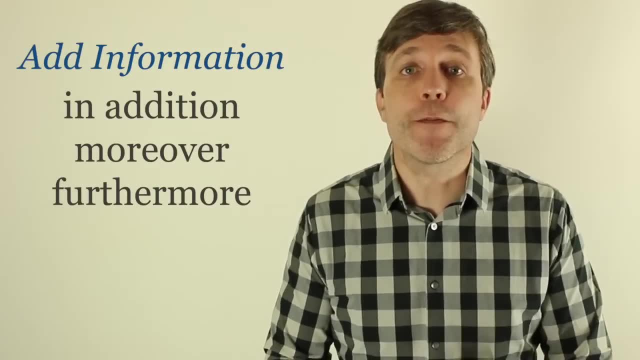 I'm adding more information and I want to emphasize it a little more. So in that case, furthermore, is entirely appropriate, Just like those words used to contrast in addition, moreover, and furthermore typically come at the beginning of a sentence, but that's not always the case. 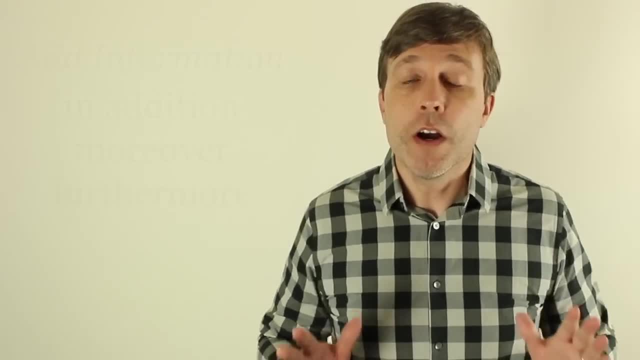 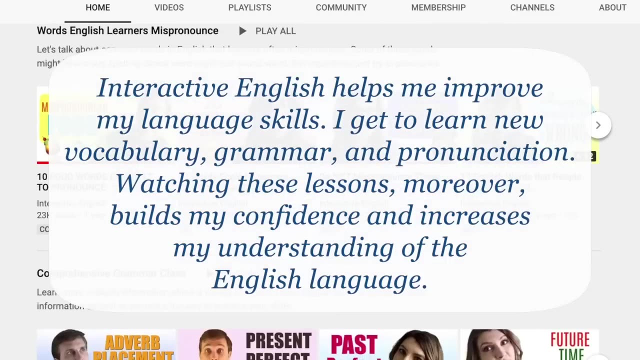 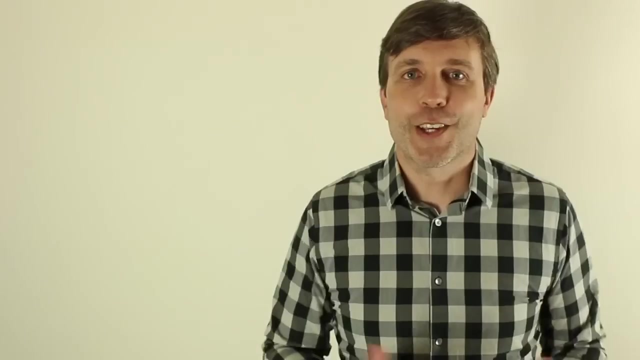 You may find them in the middle of a sentence after the subject. So Okay. Interactive English helps me improve my language skills. I get to learn new vocabulary, grammar and pronunciation. Watching these lessons, moreover, builds my confidence and increases my understanding of the English language. 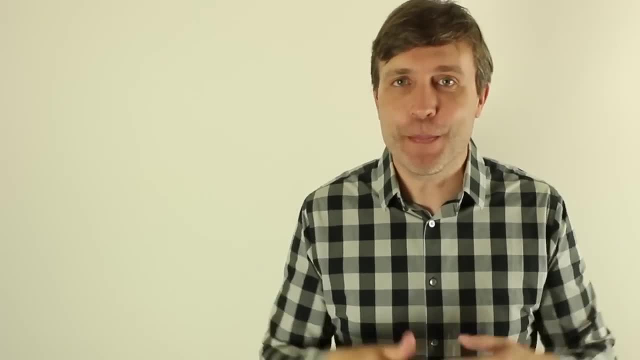 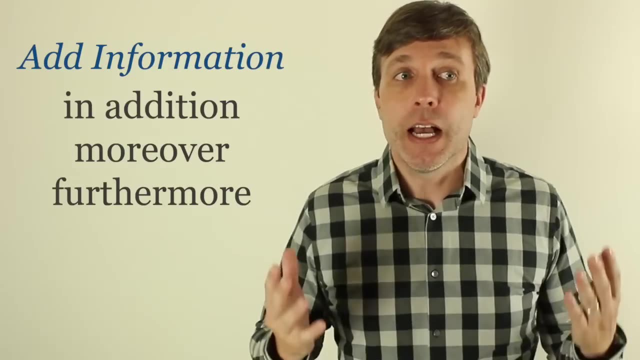 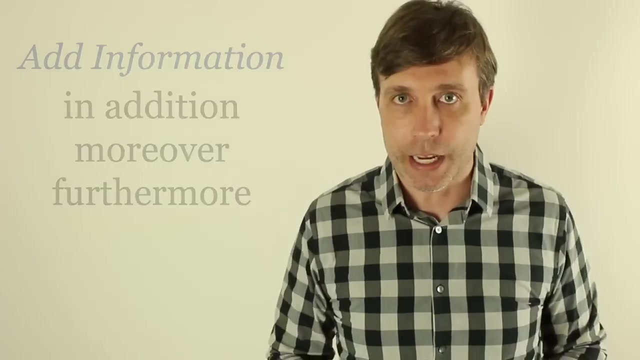 So this, this is something that I hope that you would say, but really it's just an example to show you that you can use these words in the middle of a sentence after the subject, But I I'd say that it really just it's just not as strong than if you use it at the beginning. 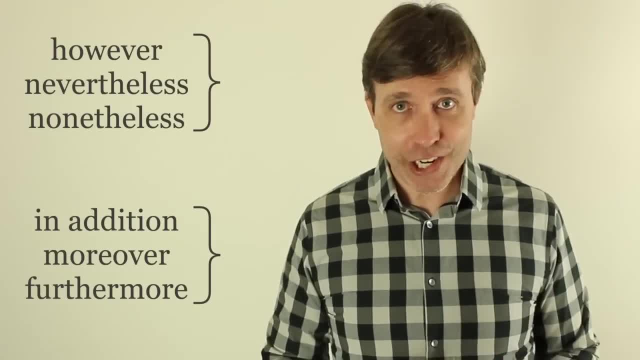 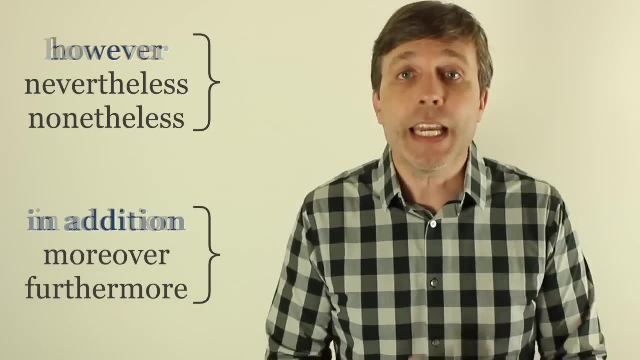 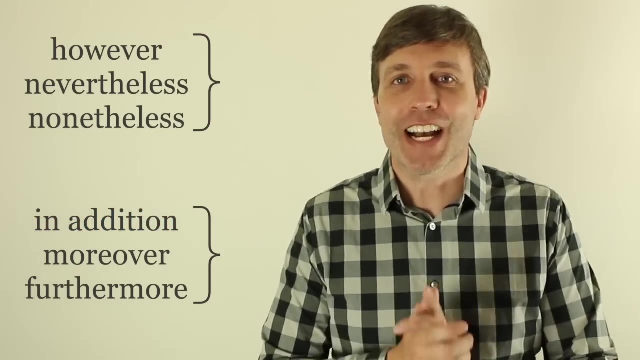 So I hope you learn something new from this lesson. In addition, please remember that, however, is most commonly used when you want to contrast two different statements and, in addition, is most commonly used when you want to add more information. Nevertheless, do not underestimate these other words, because if you want to be a bit more, 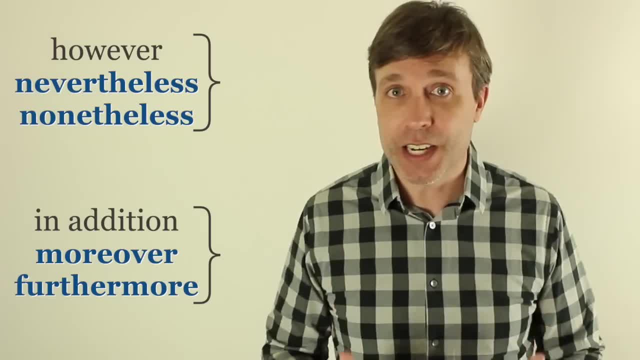 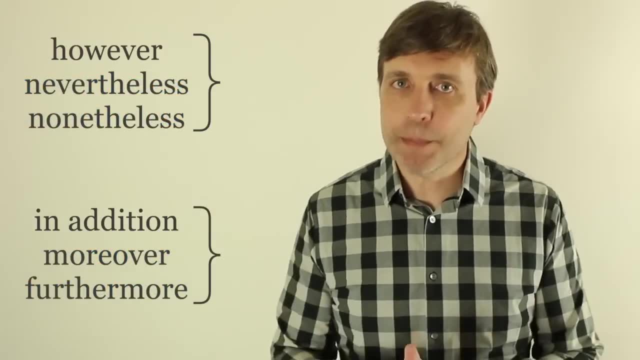 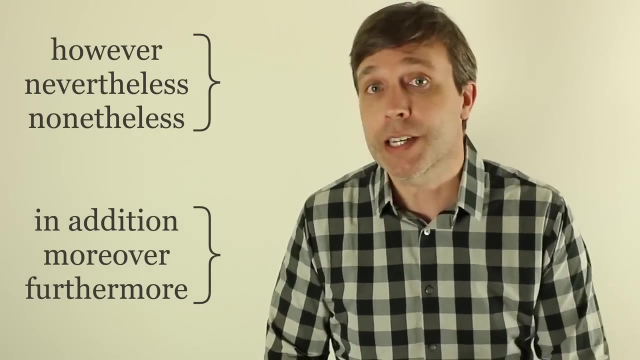 formal or you really want to emphasize that there's a difference or emphasize the additional information. That is when you should use these adverbs. Moreover, it's absolutely necessary that you continuously try to use different words. If you are, if you're doing things like giving a presentation or you're writing some important